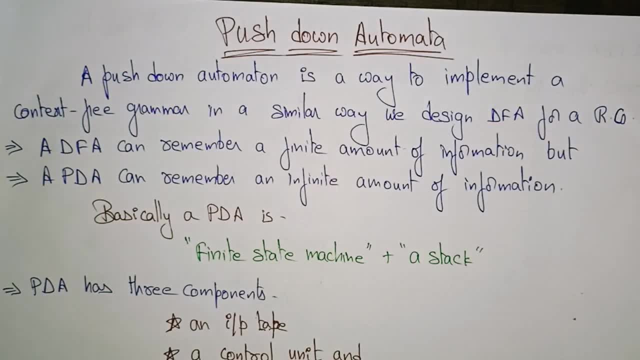 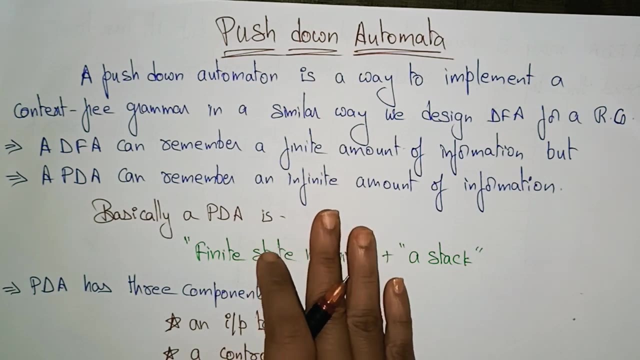 Hi students, coming to the next topic, that is, a push down automata. So far you had seen so many concepts like the deterministic finite automata, non-deterministic finite automata, context-free grammar and so many concepts you had seen. Now let's come into the push down automata. 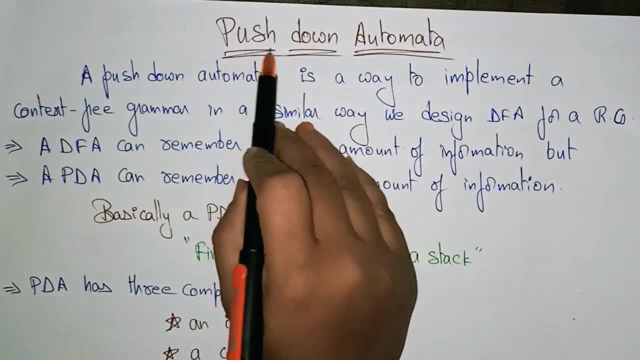 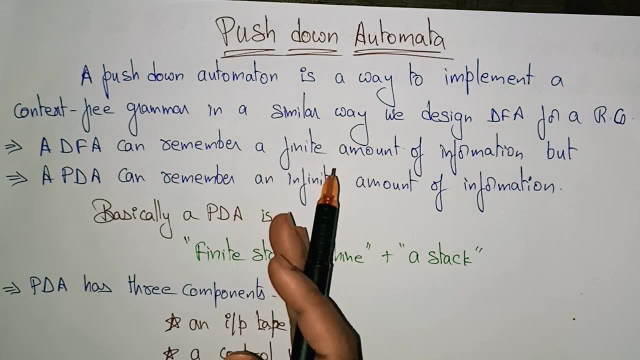 So it is asking. the name itself is saying that we push whenever you've seen the word push means means. in this we are using the concept stack. So where the terms push and pop will come, the push and pop terms will come in the stack. So in this automata we are using the concept stack. 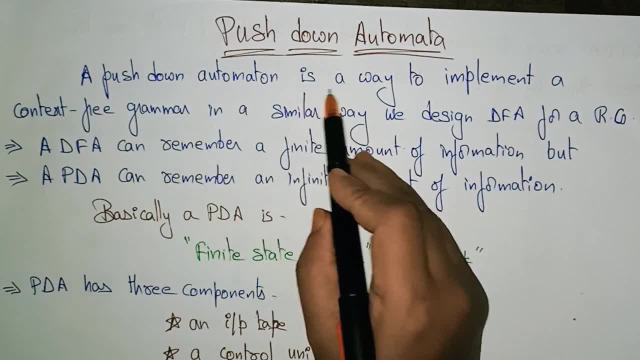 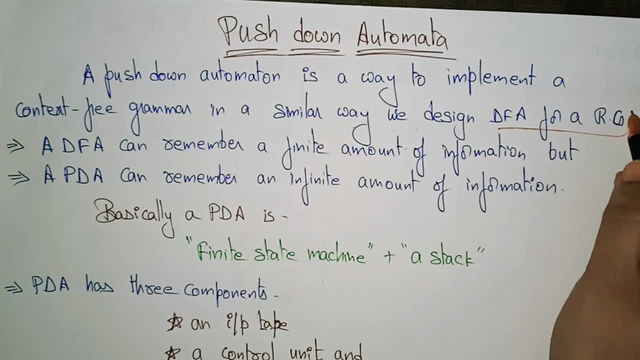 Now let's see a push down. automata is a way to implement a context-free grammar. in a similar way, we design the deterministic finite automata for regular grammars. So, whatever the deterministic finite automata is, it is a way to implement a context-free grammar. in a similar way we design. 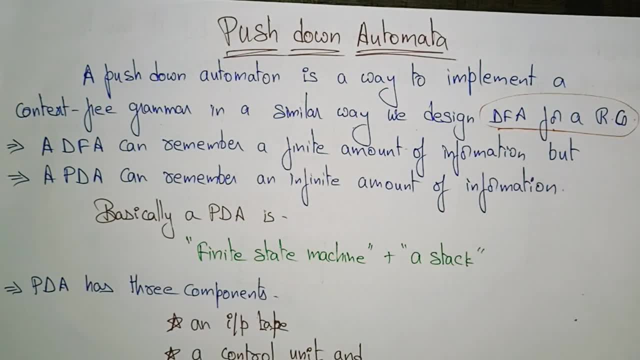 for regular grammars. For regular grammars, we are use the non-deterministic finite automata and deterministic finite automata In the same way, whatever the technique that we used for the for regular grammars to design the deterministic and non-deterministic finite automata. 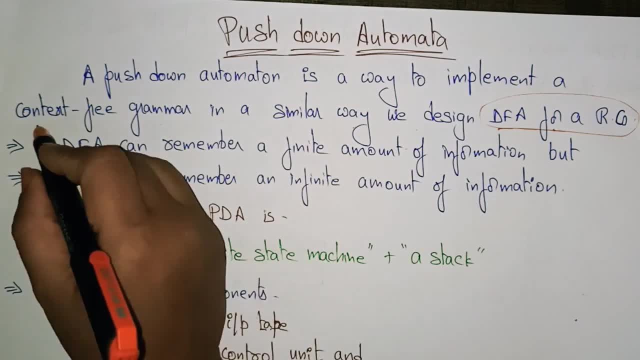 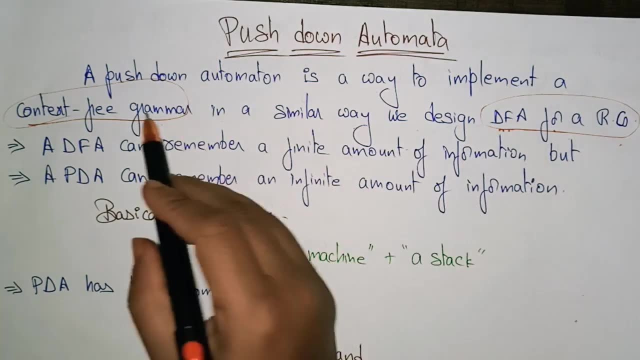 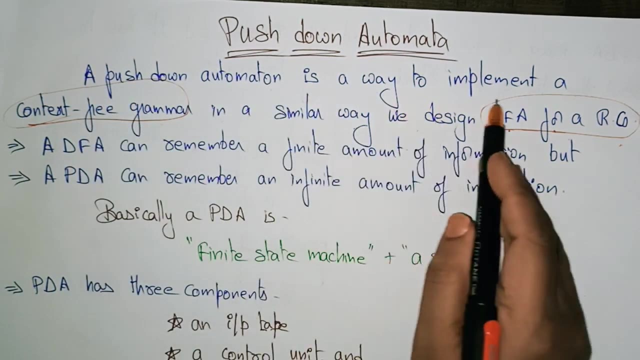 The push down automata is a one of the way to implement the context-free grammar. So NFA and DFA for regular grammars and for context-free grammar. one of the technique that we used is a push down automata. The push down automata is a way to implement the 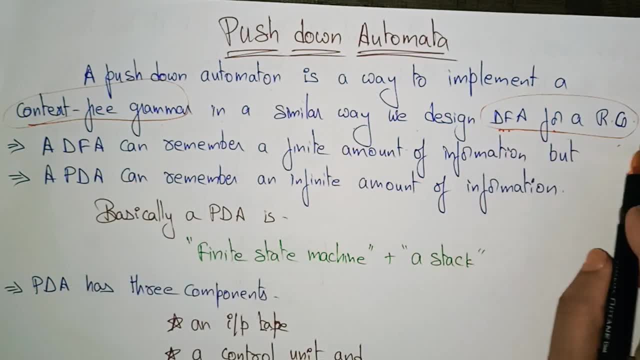 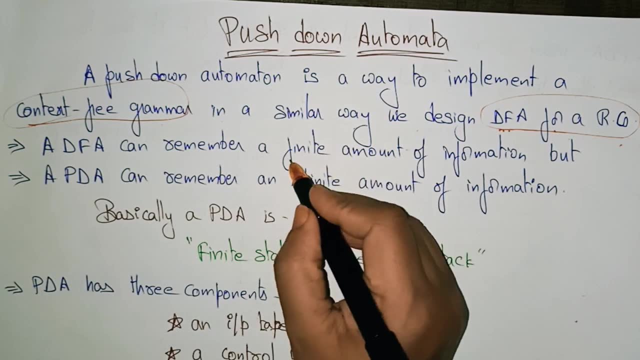 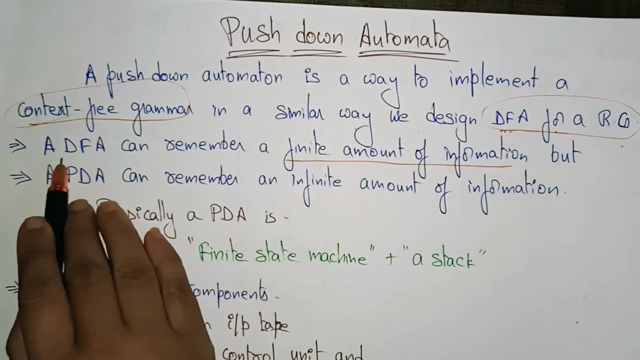 context-free grammar and NFA and DFA is a way for the regular grammars Now coming to here. a deterministic finite automata can remember a finite amount of information. The main difference between that deterministic finite automata and the push down automata is: whereas in deterministic finite 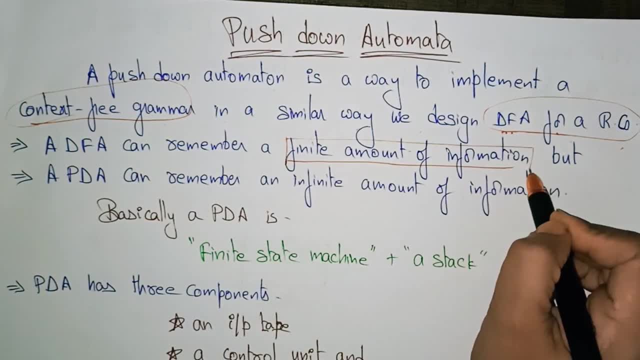 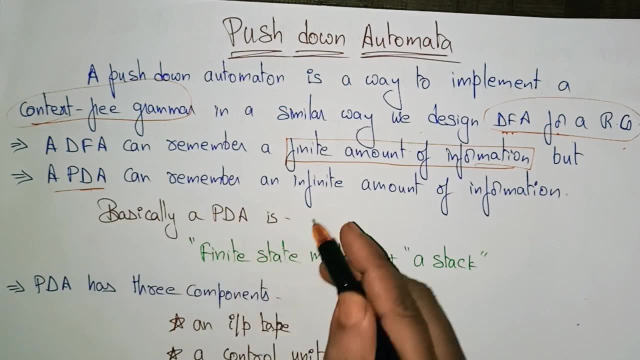 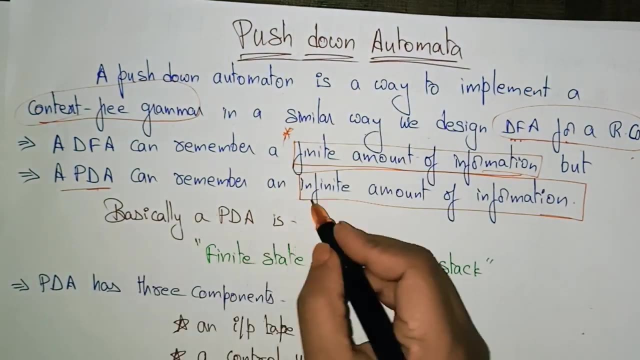 automata, it can be remembered with only the finite amount of information. only it can handle infinite amount of data, Whereas in the push down automata it can be remembered as infinite amount of information. So this is the main difference. This is for finite automata and PDA. 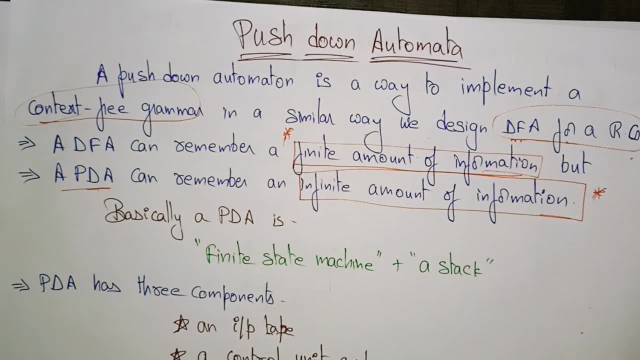 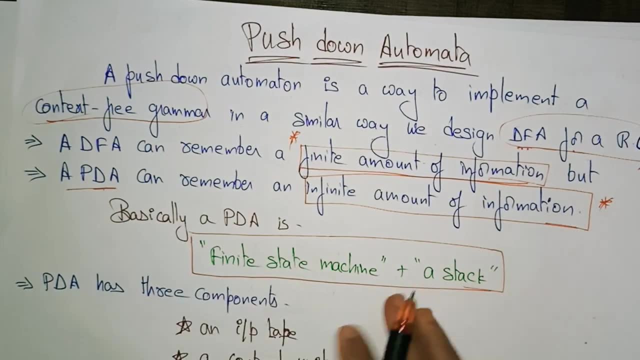 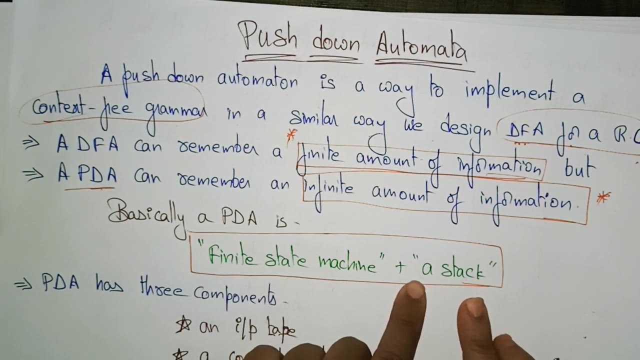 is for infinite amount of information, So basically a PDA. the push down automata is a finite state machine plus stack. So the finite state machine constraint that is only deterministic: finite automata plus stack. You call it as a PDA. Okay, The basically push down automata is a finite state machine plus a stack. 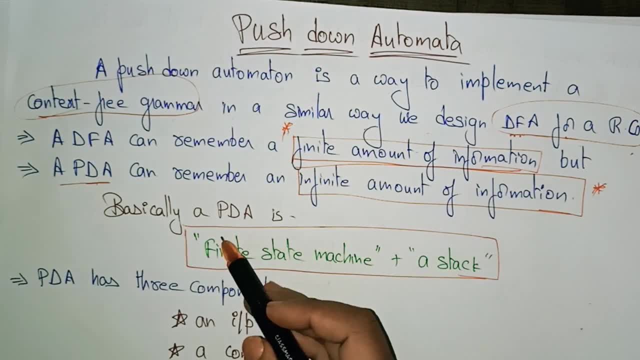 Because why it is. we are using stack to store the infinite amount of data, So the stack can handle the infinite amount of data. means whenever the data we are pushed, if you want to accept the stack, the data has to be popped. So then, always after the completion of the instruction, always the stack. 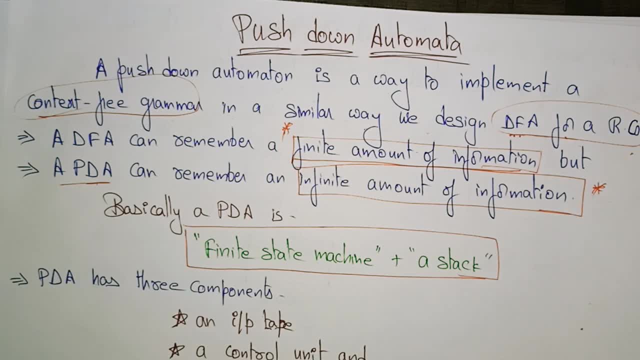 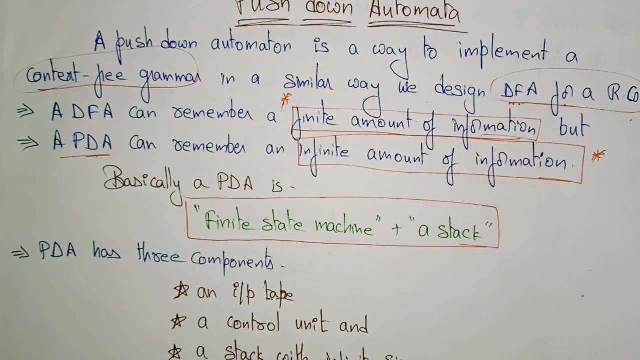 becomes empty. Whenever it is empty, you can store more amount of data. So you can store more amount of data in that right. So that's why we call it as an infinite amount of information can be handled by the push down automata because of the stack, Because of the help of the stack. So PDA has three. 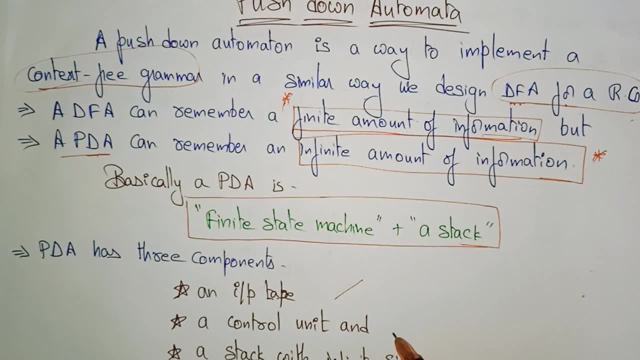 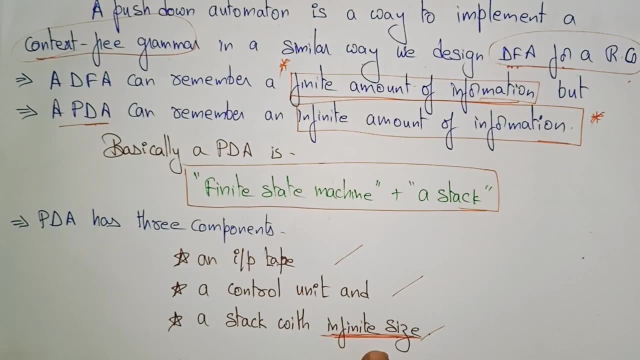 components. Mainly three components will be there: The input tape, control unit and a stack with infinite size. So remember this: a stack with infinite size. So what are the three components that push down automata, consisting of Input tape, the input information unit and the stack with. 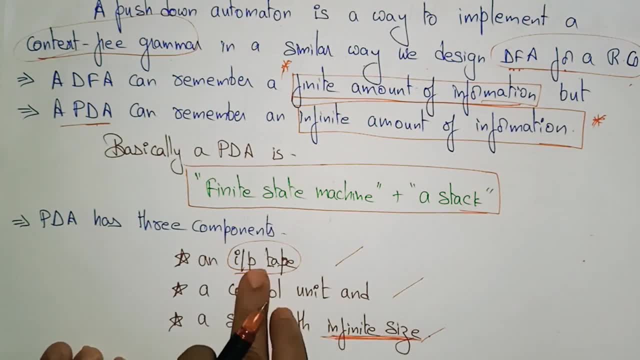 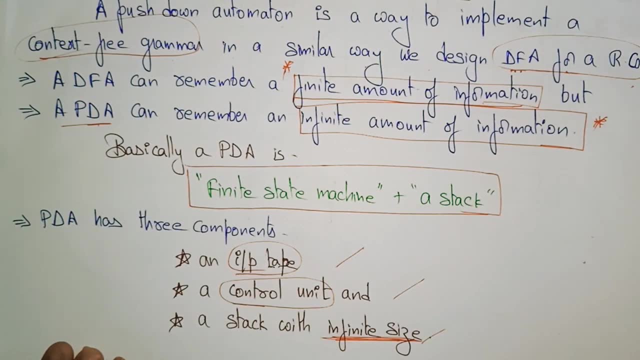 information that will be stored on the input tape. That is, unread data is stored on the input tape and the control unit which is controlling to transfer the data from input tape to the stack, and a stack with infinite size. Let's see the diagram to understand these three components. 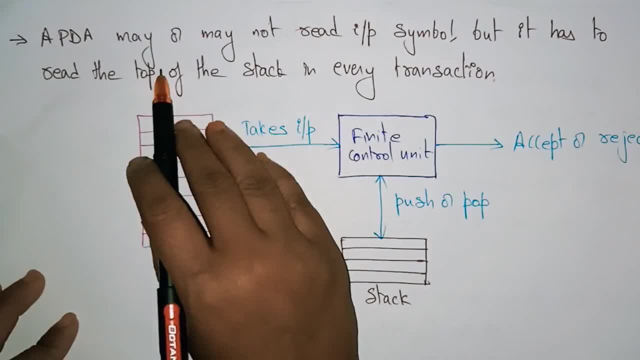 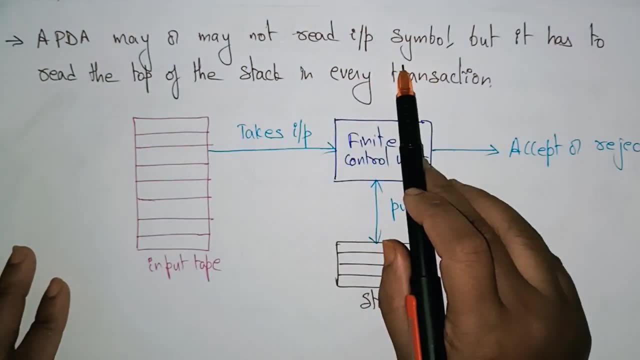 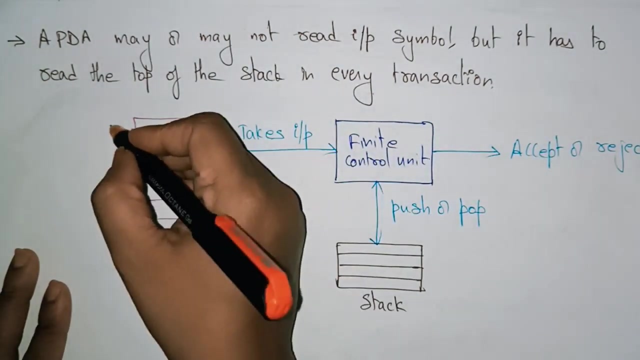 Okay, So this is the diagram you can see. here The PDA may or may not read input symbol. So here the PDA may or may not read the input symbol, But it has to read the top of the stack in every transition. So whatever the elements that are, 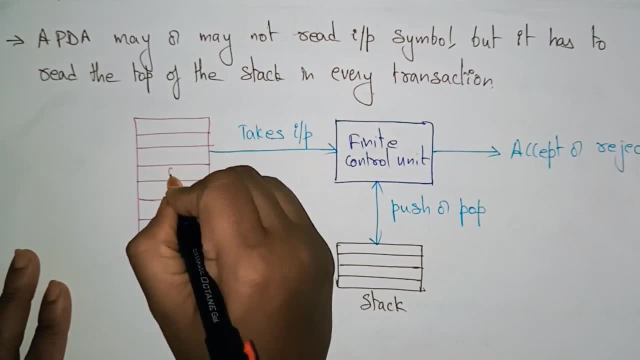 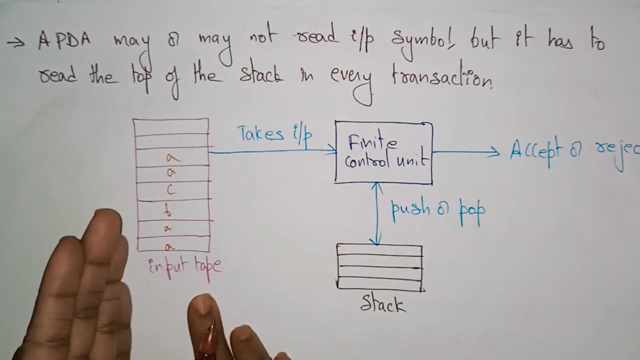 present in the input. let us take A, A, B, C, A A, like that. Some elements are there in input tape. Okay, Input tape. So here the PDA may or may not read input symbols, It may or may not read the.